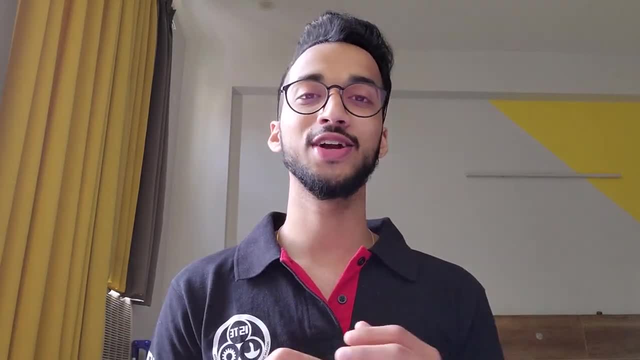 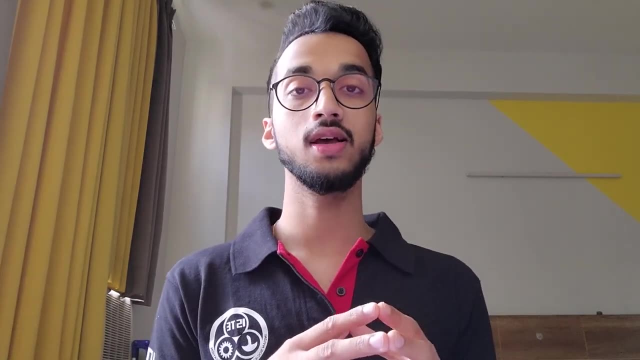 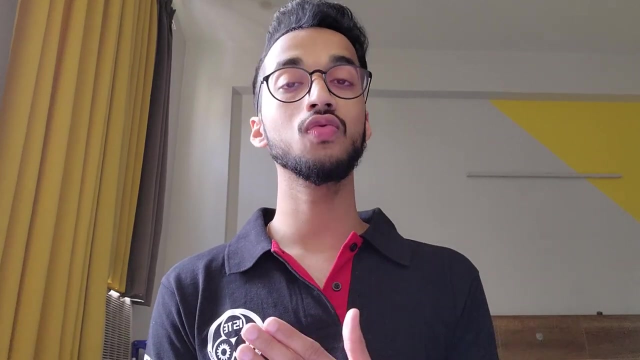 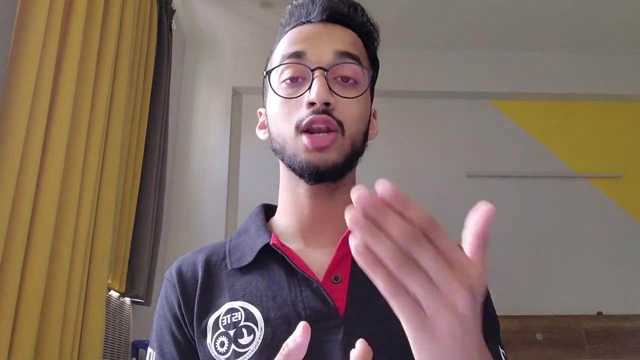 Hello everyone, my name is Nachikita and welcome back to another video. In this video I'm going to be talking about what I do as a computer vision engineer. This is a field which has been rising lately: The field of AI and video. AI is getting a lot of hype and there is a lot of demand for computer vision engineers who are good at what they do. So as a fresher or as someone who has not worked in this field, there could be a lot of doubts you would have So as to what would someone actually do in a future video. 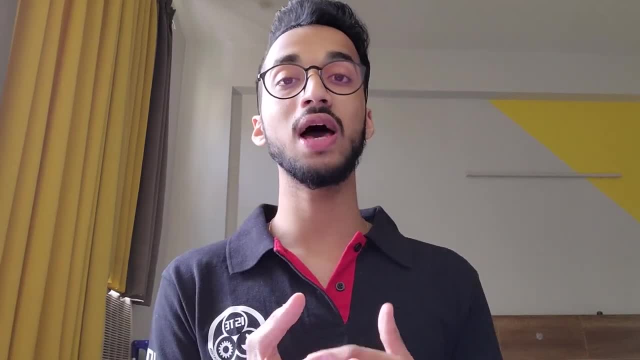 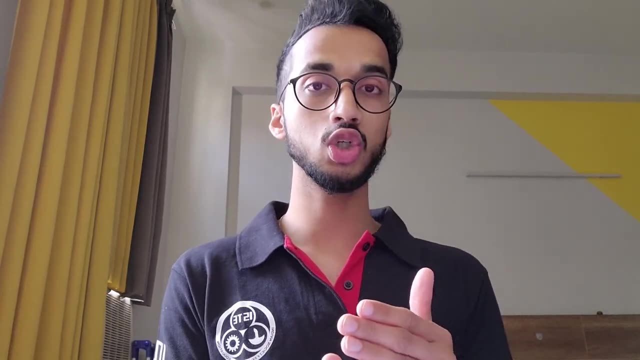 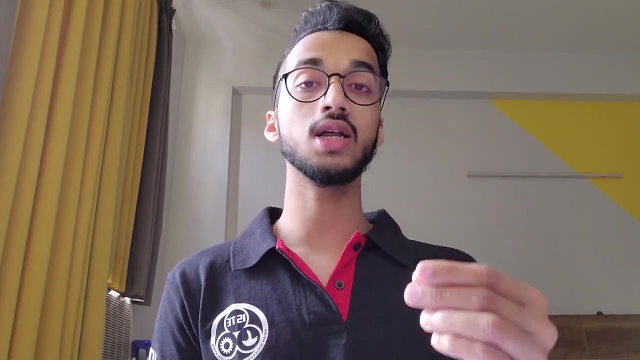 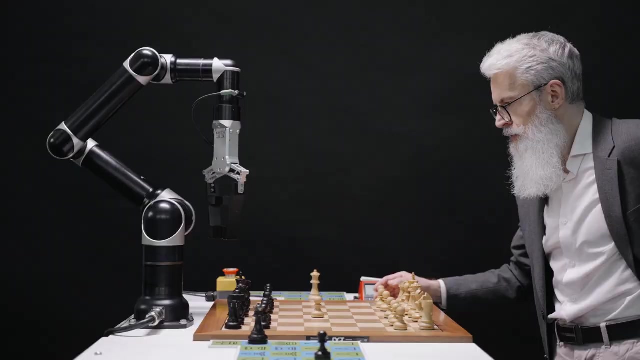 What would be the typical requirements, What could be the typical responsibilities. So I'm going to be talking about what computer vision is, what I do as a computer vision engineer, what would be the typical skill sets required for this job and some basic tips that can help you get started in this field as well. So, to start with, what's computer vision? Computer vision is a field of science which will basically help a camera interpret video the same way as a human does. 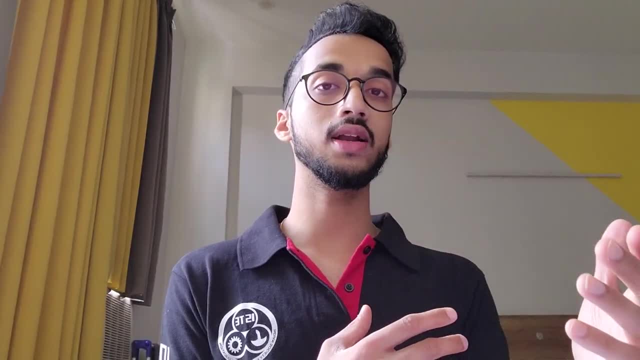 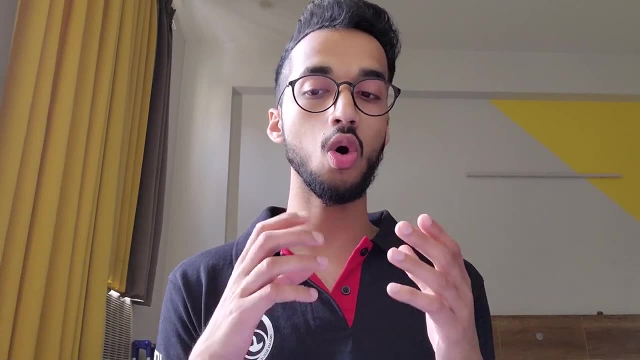 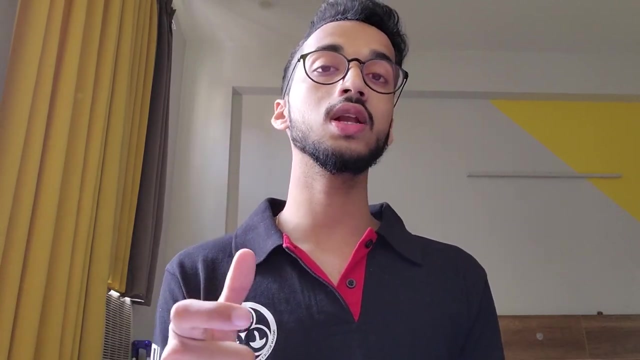 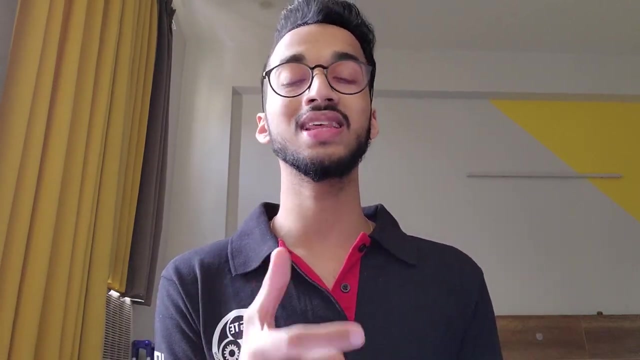 So, for example, if you show me a photo of a dog or a cat, I can understand what this is, what the context is, But when a computer sees this image, when a computer sees this image, all it sees is pixels. It does not have any understanding of the image. So building AI algorithms working on image processing, so that cameras can now perceive images the same way humans do, is what computer vision is all about. There are different forms of this. There are different uses of this. So a self-driving car. 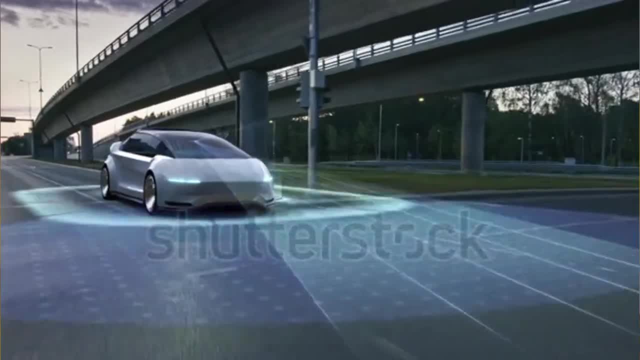 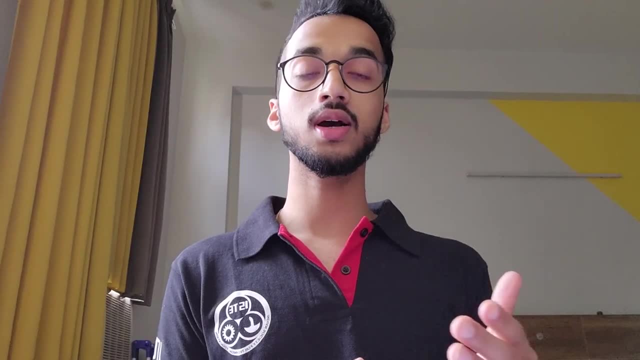 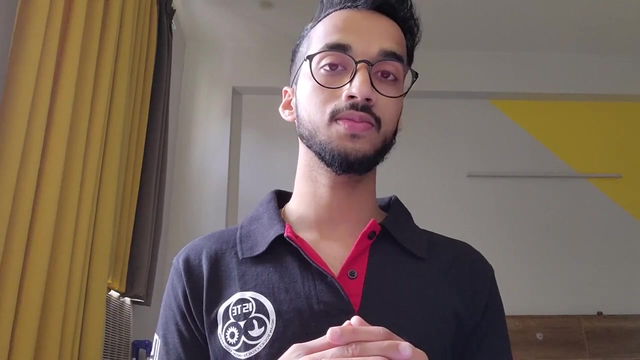 would be one application of a computer vision problems, Whereas a car is using a camera to interpret roads the way humans do. So, depending on what company you're working in, what the main product is, there could be different ways- or of how you're using computer vision. 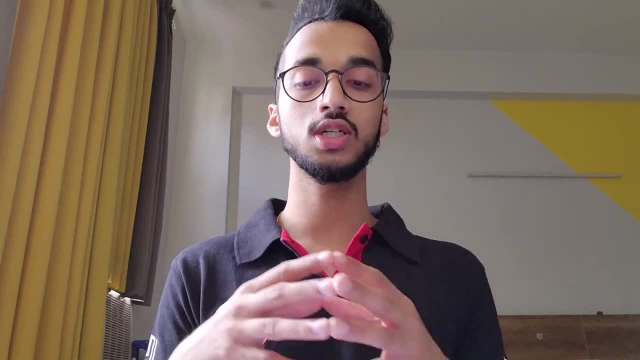 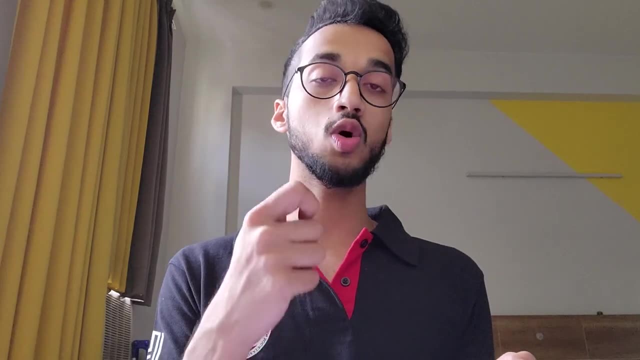 So when I talk about my specific role, I work at Abyros, which is a video AI operating system and marketplace. So like you have Android and like you have iPhone, Abyros is an operating system, computer vision application, so like you have a play store or an app store on. 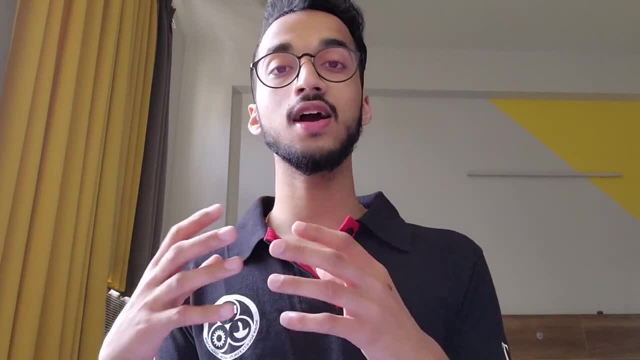 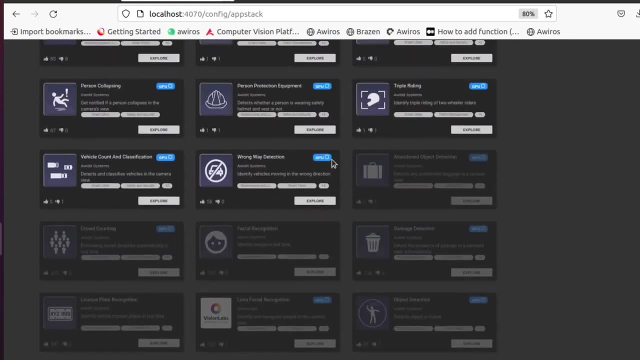 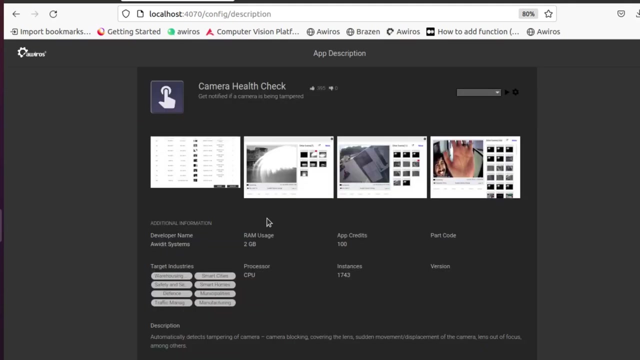 your phones, we have the equivalent of that which we call as the avirose app. stack right. this is a compilation of video AI application that any customer would need and, as a computer vision engineer, my job is to build these applications for the end customer. so, to give you an example, we have an. 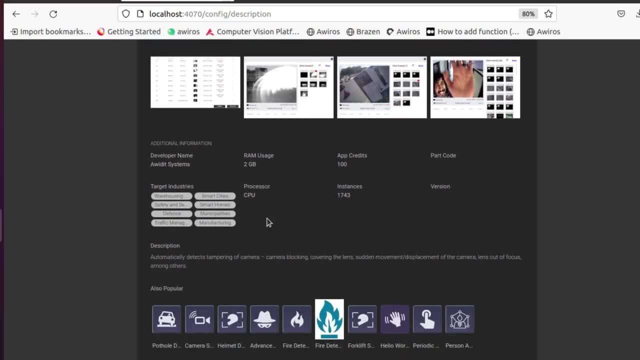 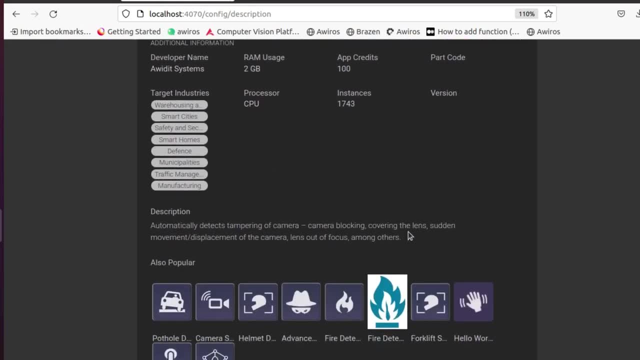 application for camera health check. so I'll only stick to the. I'll only stick to one application for now and I'll show you what the process is. so let's say we get a requirement from a customer that they need a camera health check application, which basically means that if a camera is being tampered, right if 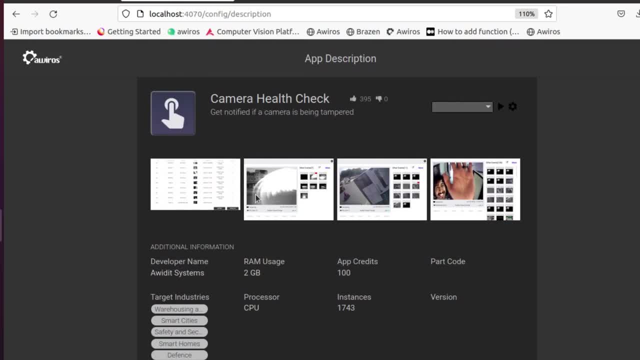 someone is blocking the camera view- and, let's say, a robber at a bank, right. or if someone is changing the camera view, flashing a light on to it, then basically the user should get a notification. so different applications have like. that is what we are supposed to build now, based on this. 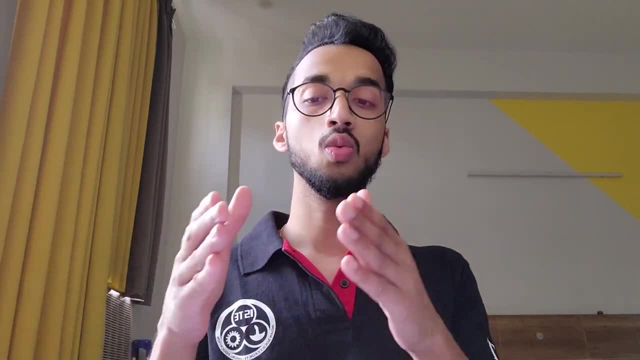 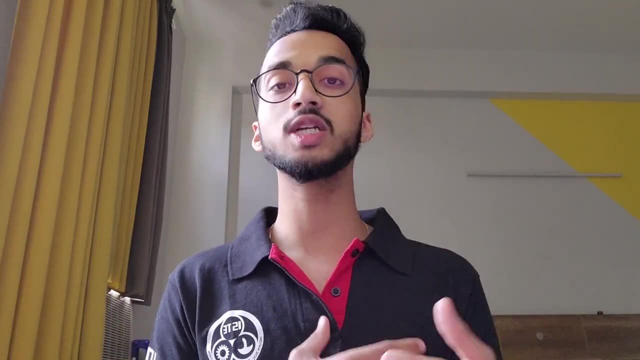 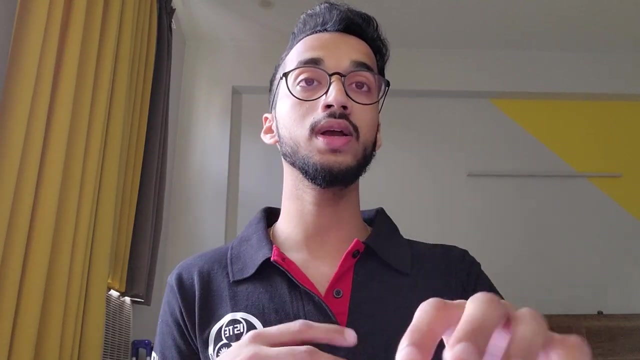 application. we have to work on pre-processing of the data, working on different data augmentation tricks, taking care of data imbalance and then building AI models or image processing algorithms that can help accomplish the given task. so just to give you an example of what my end goal would be, it is to get a production. 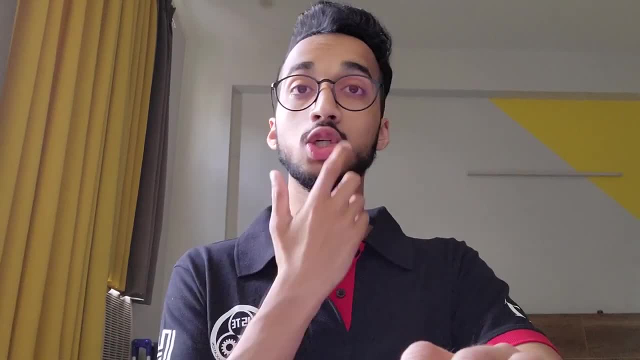 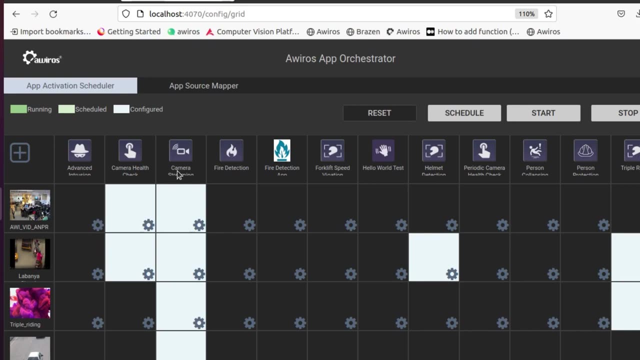 ready application which a user can use right. just to give you an example, to show you how it happens in practice at my company, this is, this page, is what we call as the avirose app stack app orchestrator, wherein the rows at the top, the row at the top which you're- 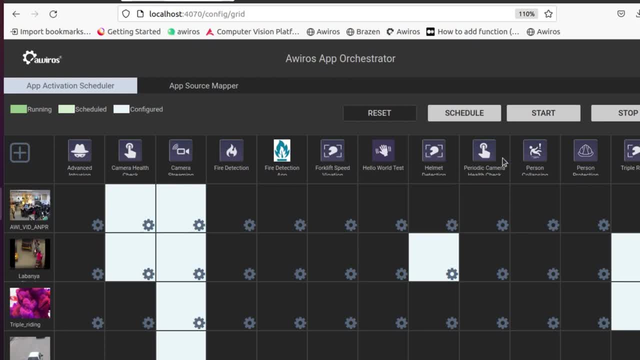 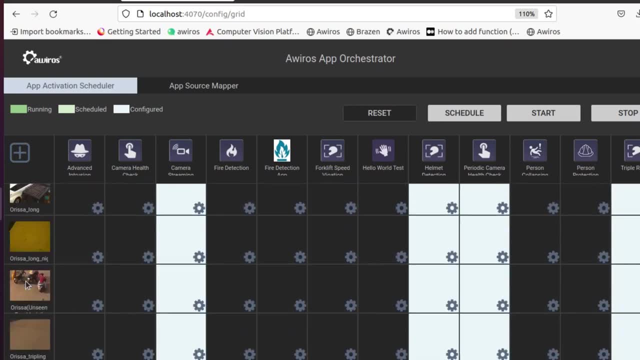 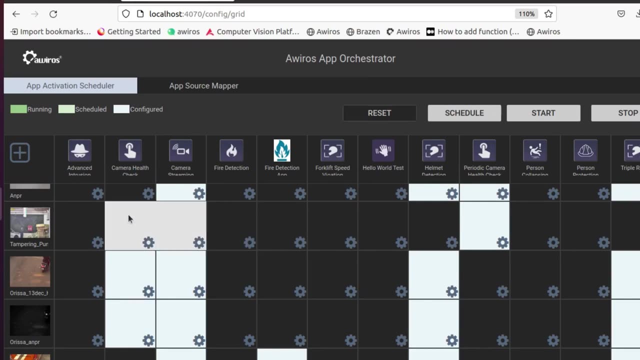 seeing represents different video AI applications and the column at the left represents different videos or camera sources. and the way you run a video AI application as a user is you select the corresponding cells which you want to run for that particular application. so the cells I selected map to a camera. 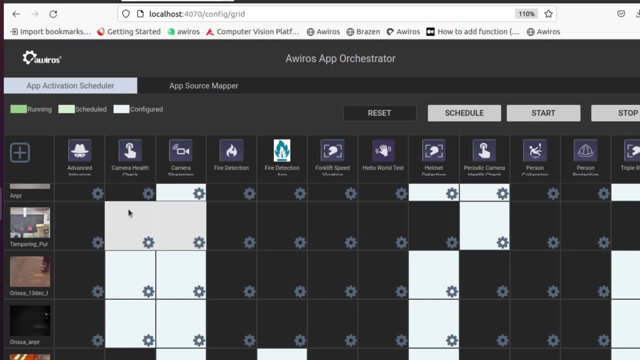 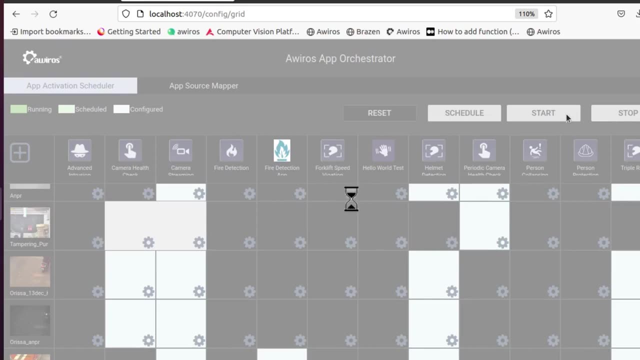 streaming and camera health check application which will run on a particular video source, in this case. so the job is: some user would select these cells and they click on the start button and in the backend the frames from the camera would come to my algorithm. the algorithm will process these frames and then make sure. 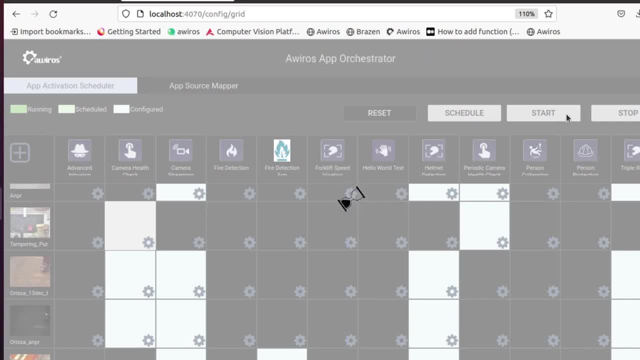 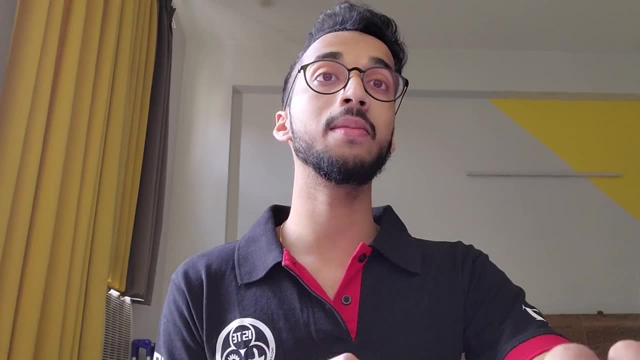 that the camera health check application works as desired. so the end result is that whenever the user runs these applications, he should get notifications whenever the camera is being tampered. so let me give you a little bit context. so let me give you a little bit context, right? so whenever I run an application, 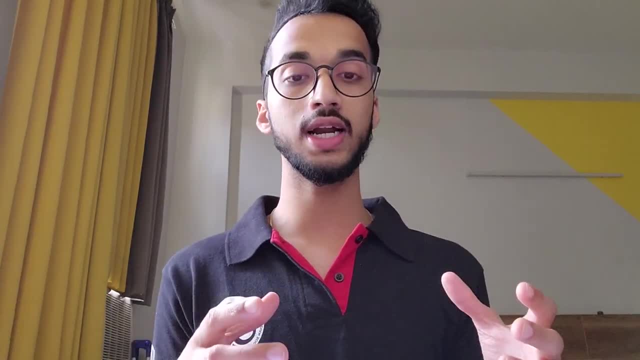 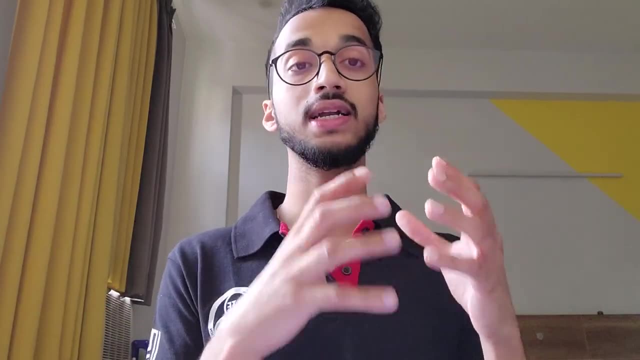 whenever I get a problem like this, we have some data set that we work with right. the data set can be acquired online from available data sets that could be synthetic generated data sets, that could be data set which you get from the client or you manually generate yourself using a camera, right. 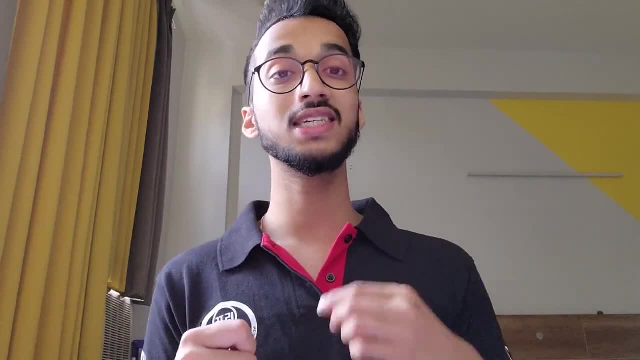 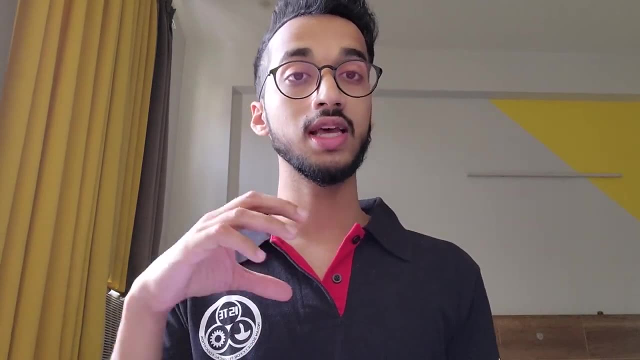 so what I had done is I had taken a particular camera and I had simulated various instances of a person tampering the camera. so if you have a different video AI application, there is going to be a different process of generating video scenarios for that particular problem. so this: 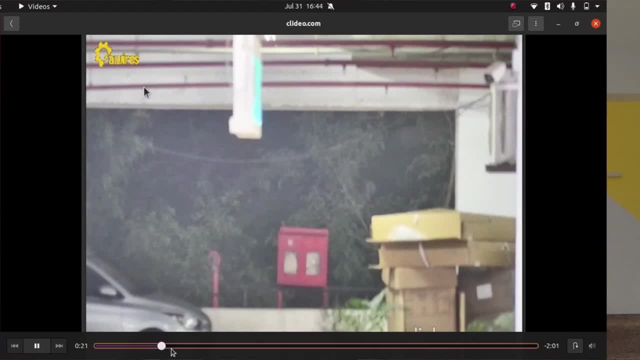 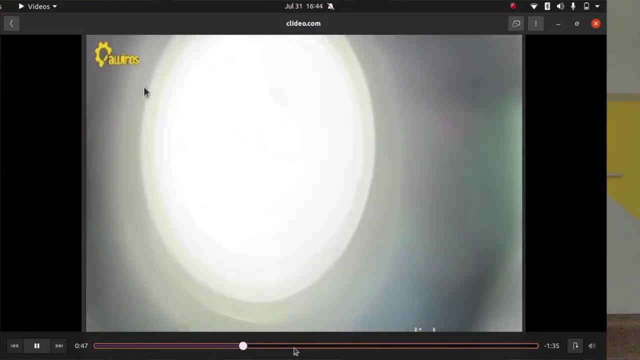 is the camera stream of the camera I had used and I went into the field of view and blocked the camera. as you can see, right about now I am covering the camera with my hand and I do different kinds of tampering. right now I'm flashing a light onto the camera- different things that a typical intruder. 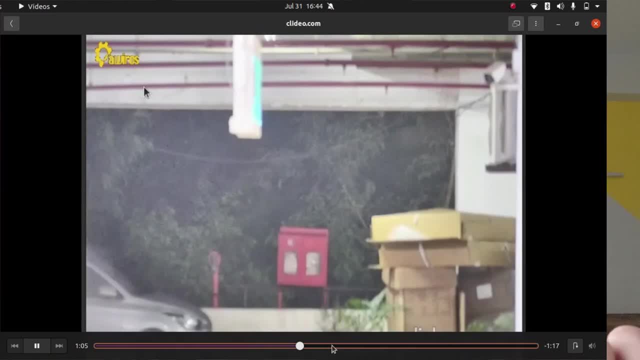 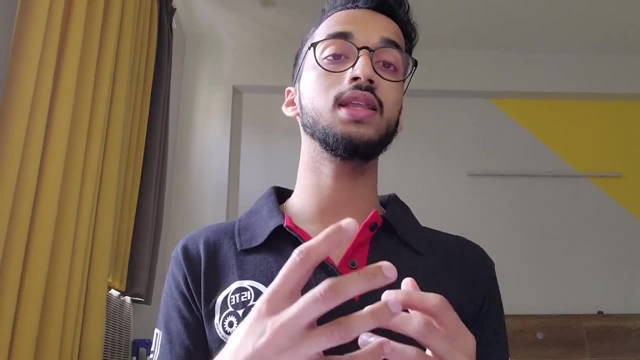 would do to block the camera right or covering the camera with a cloth or just completely moving the camera onto a table or something like that. so I had used a camera stream of the camera and I went into a different field of view, right? so this video served as a test video, basically after I'd made the 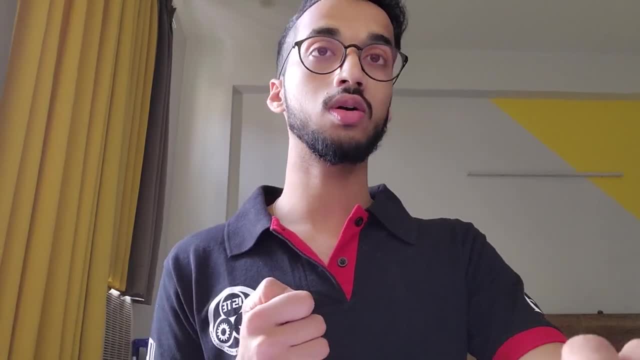 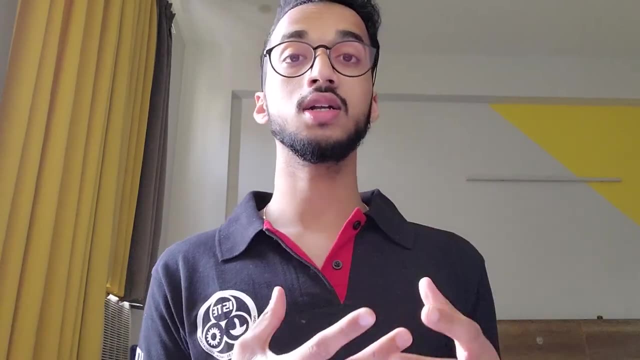 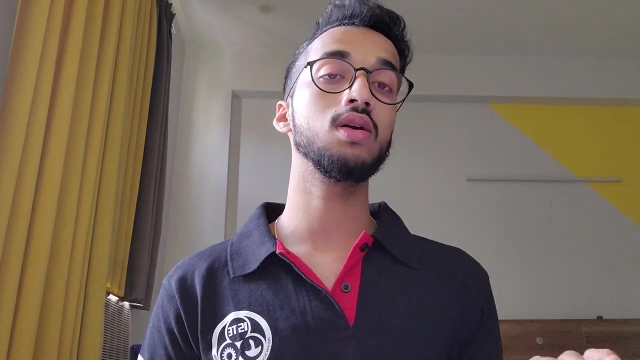 algorithm just to test if it works as desired or not. so the end result is: you get the camera stream, you run your algorithm and it gets desired results. these are some notification which come on the platform, right? so the engineering part of that is something which I which I'm not discussing how it. 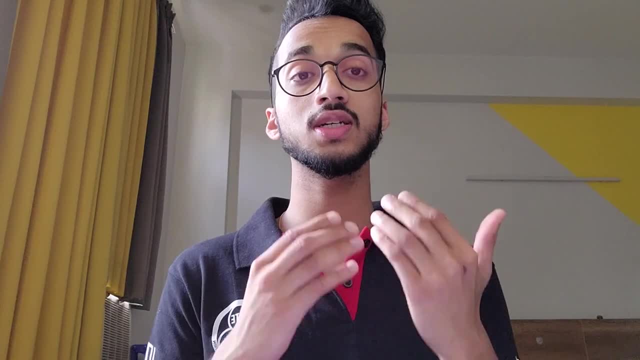 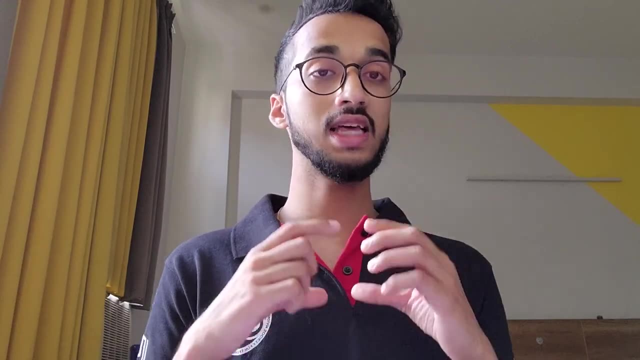 actually happens in the back end, how I get a frame, how it's processed, how it goes back into the front end. but the main point is the camera right. I get the camera stream, I process that. there is a way of pushing that alerts back onto the UI and the end user will get notified, for example, in this: 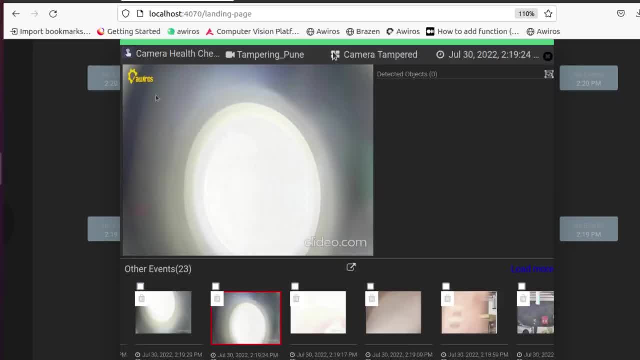 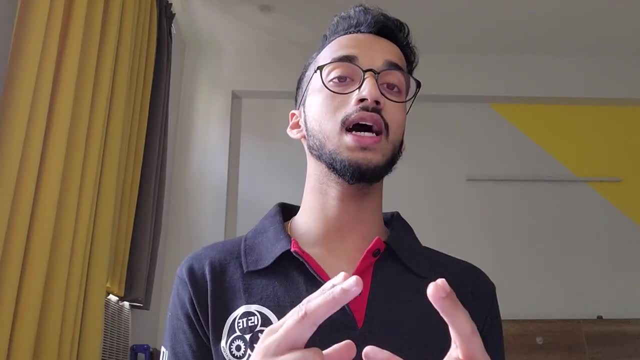 particular screenshot I can see the camera view is being blocked and it says: over here the camera is tampered, right? so this is the end result, right? so this was just one example of an application. we have different applications for different use cases, for different customers as a computer vision. 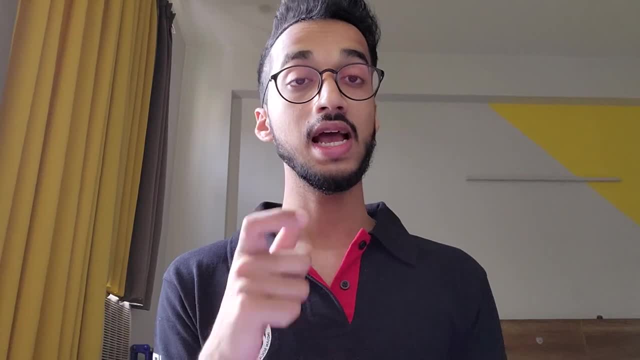 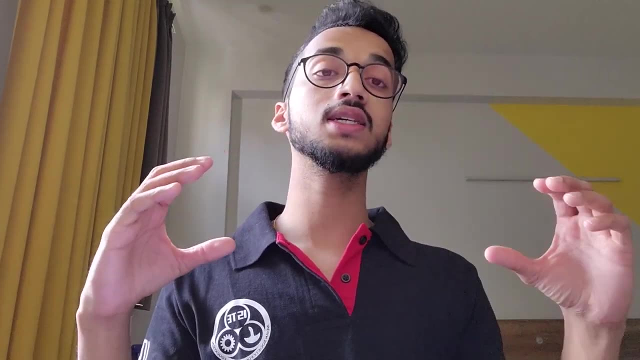 engineer. our job is that we make the video AI application and we make the video AI application and then push that into production and make it scalable. so these two parts- making a video AI app and making it scalable- requires two different skills, that which I'll talk about when I talk. 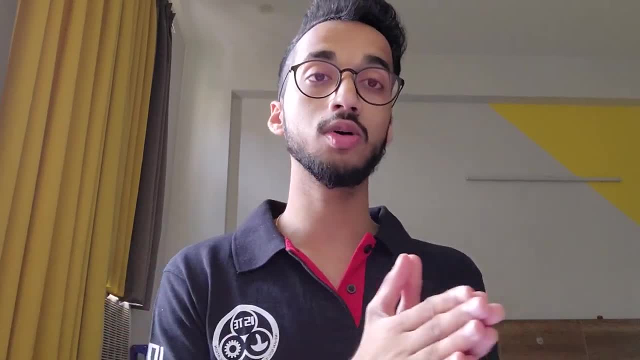 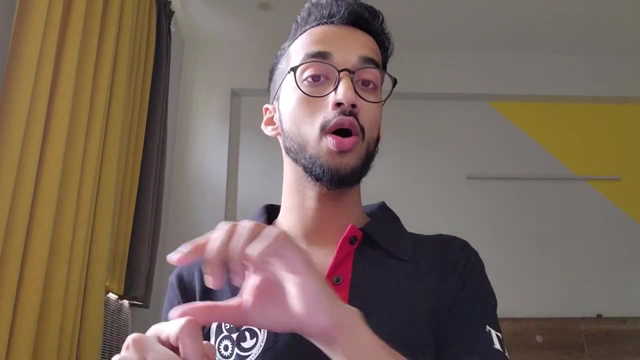 about making the video AI application right. this could be for any purpose. let's say you are using a camera to read the number plate of a car, or you're using the camera to count the number of boxes on a conveyor belt in a manufacturing factory- right. so the application could be anything. as an engineer 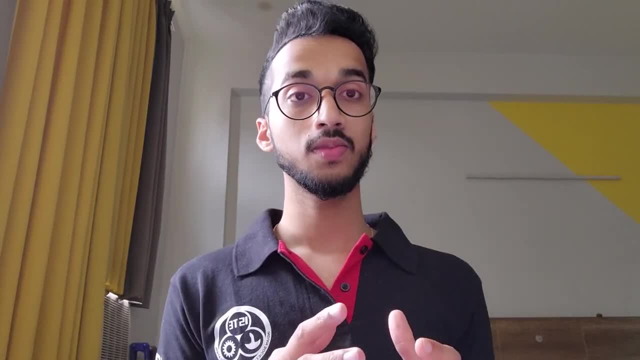 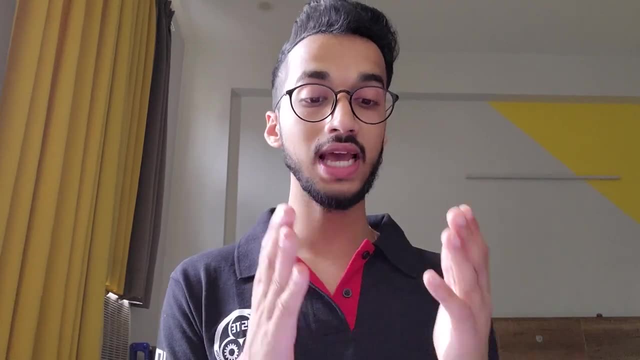 your task would be following that process, and then you can make the video AI application, and then you can make the video AI application also, and then you go back to the home page is the right way where you can make the video AI application. okay, so with this application, the animation- you can make the 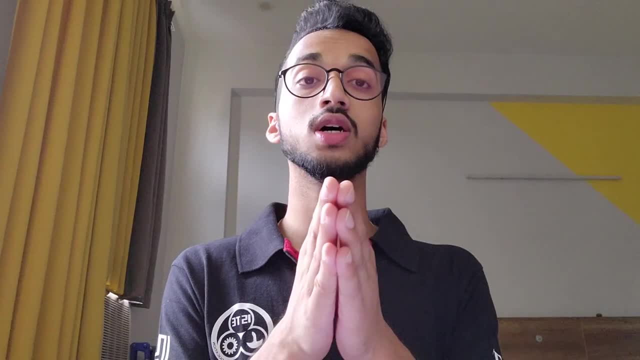 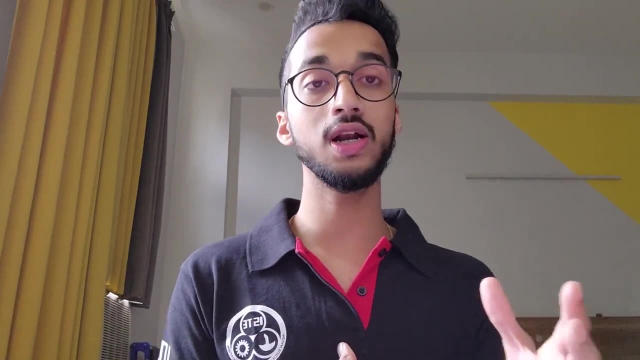 video AI application and then you need to create some kind of a data structure, right? so let's say that we wanted to make a video AI application for a computer and we need to create a model to actually make it work, because we're not using any other arbeiten. the advantage is you're not. 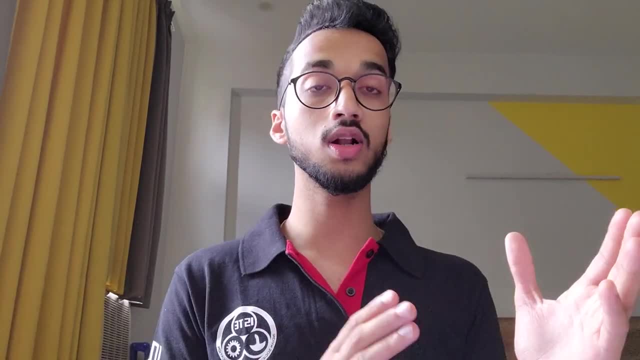 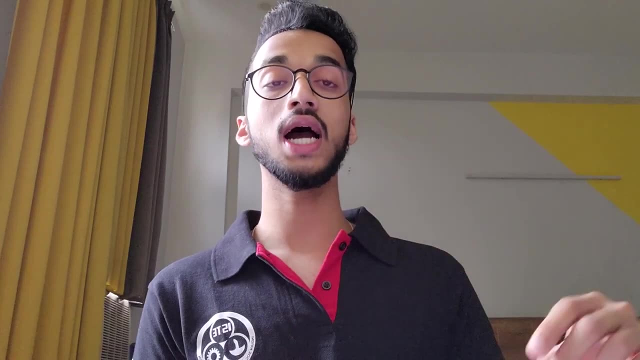 gonna have to go through the actual process, right. so basically, you're just gonna make a video, for to make the video, AI application right. so you just need to create a model for that. so this is where the get results on that. once that's done, the next thing is pushing it into production, which requires 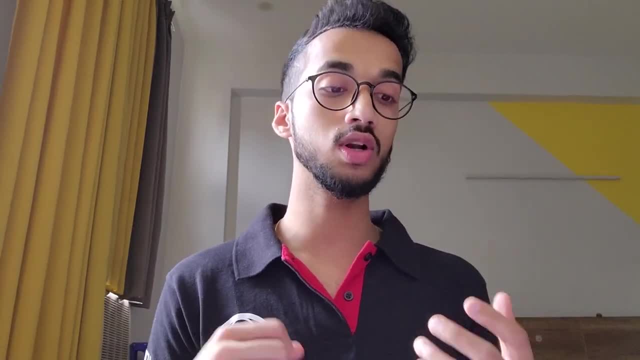 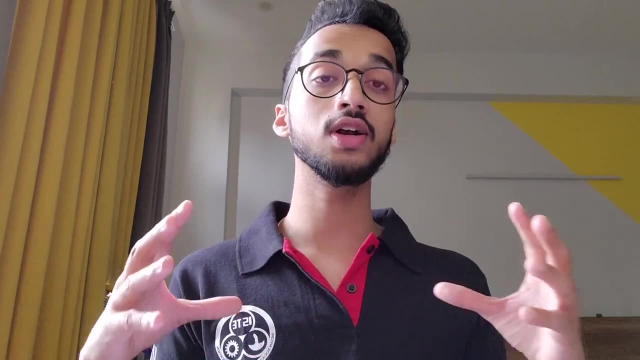 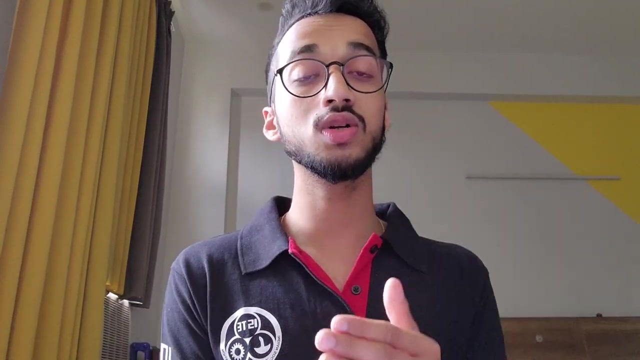 different aspects, different skill sets of software engineering. for example, if i talk about my application right. once i build an application, we have to make sure that it's compatible with different software and harvard architectures. it's running on cpu versus gpu. we have to containerize it, monitor the usage. how much ram is it consuming? how much gpu course is consuming? 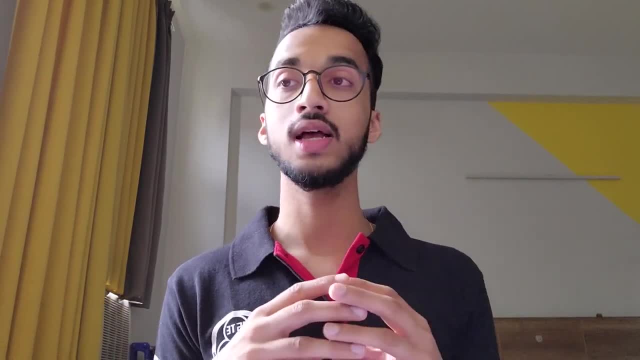 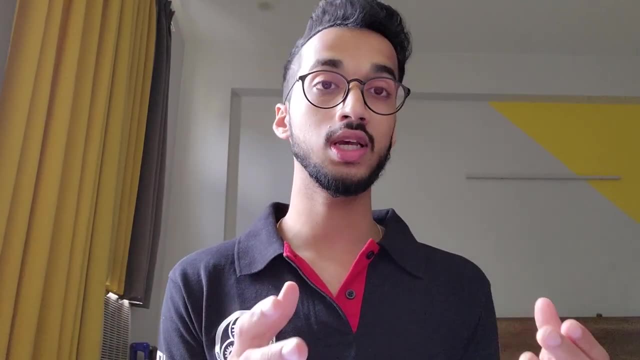 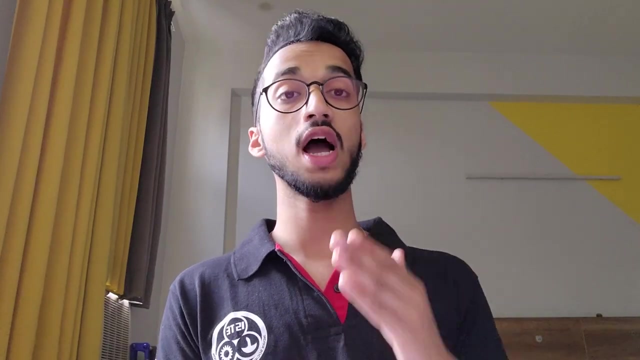 load balancing on different servers to make sure that the customer is able to use the application with the minimum amount of processing and minimum amount of cost in turn. right, so now let's talk about. what are the requirements, what skill sets you need to have if you want to work as a computer vision engineer, if you're interested in the field of video, ai. 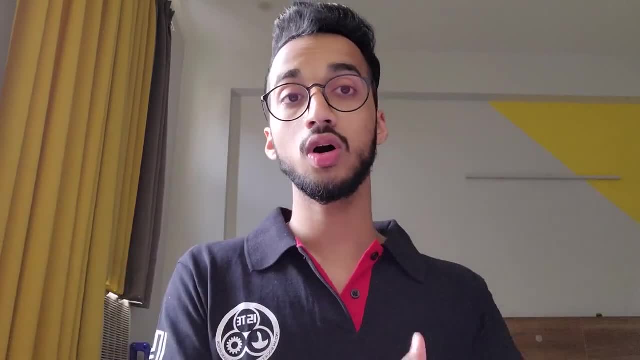 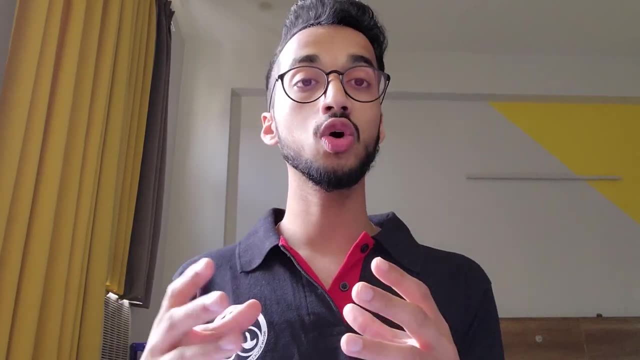 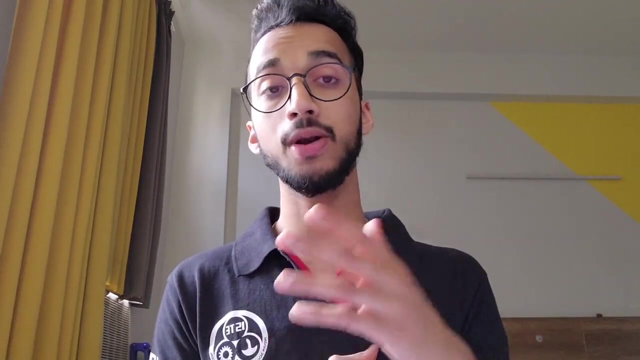 yourself. again, it differs company to company based on the product they are building. but the general skill set is: you need to have basic software engineering skills. you need to have basic of machine learning, deep learning and computer vision. you need to be good at programming. again, the programming language is: it could be again different company to company, right, but 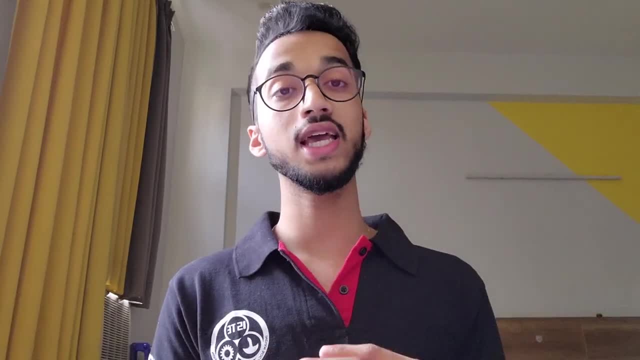 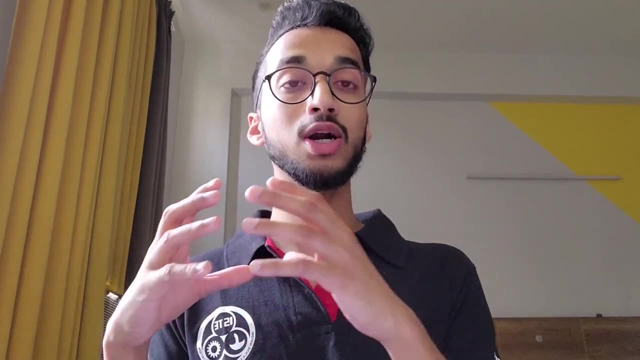 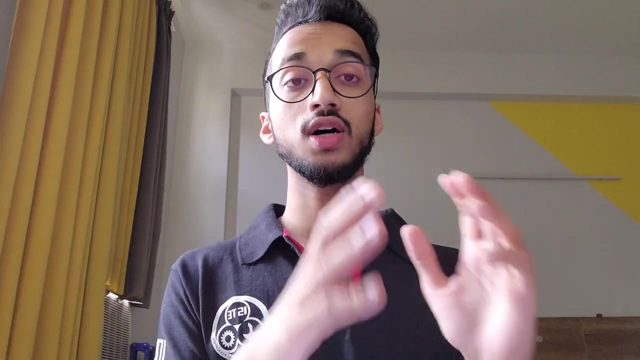 it's normally either python or c++. in my given role we need both. in my given role we use both. so, for example, we train models in python, but to ship that into production we need to integrate that with c++ to optimize speed. so i would say: first pick one program. 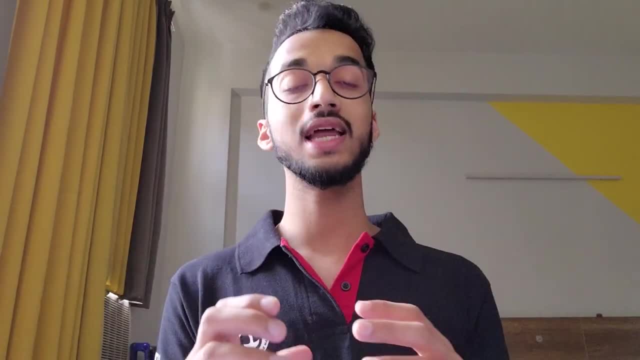 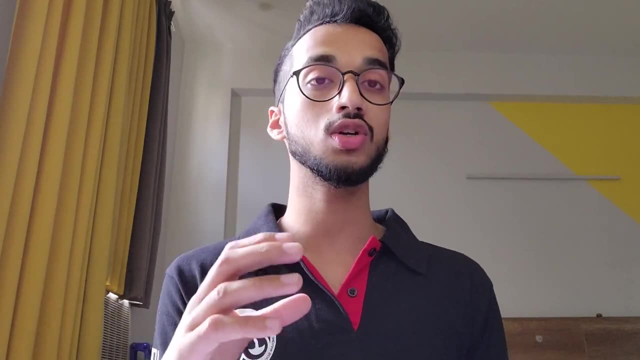 language, let's say python. if you become proficient in that, then you can start working on c++ as well. most companies, if you're good at one programming language, you're good at algorithms, you're good at data structures, in that then they would give you a chance, because picking up another programming 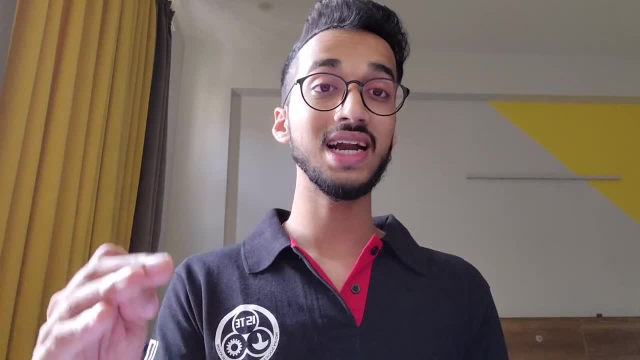 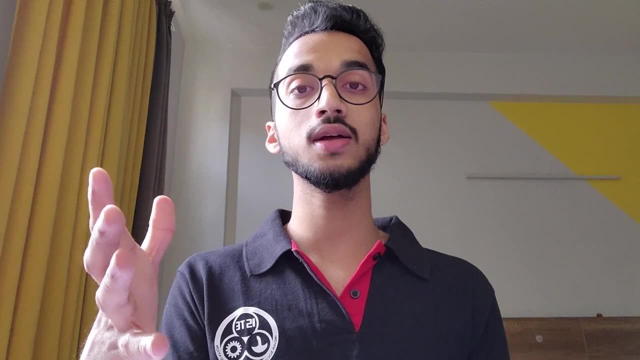 language is not that hard if you're good at one. so, understanding of programming languages, basics of data structures: no one will ask you to invert a binary tree, typically in startups. but they will expect good knowledge of the basics data structures and they will ask you to invert a binary tree. 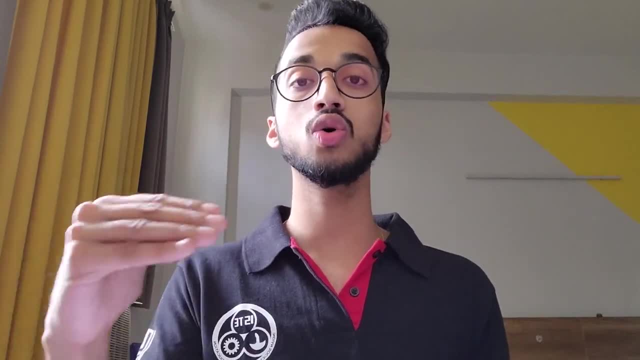 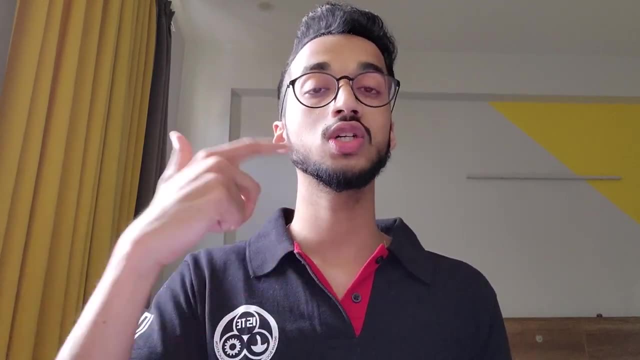 so you can get good knowledge of the basic data structures, the inbuilt data structures of different languages and how to access and manipulate them as well. another important thing is knowledge of deep learning libraries like tensorflow, pythons, darknet and opencv. right. these are libraries that 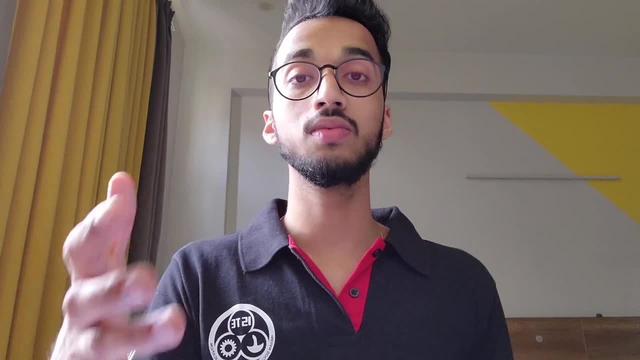 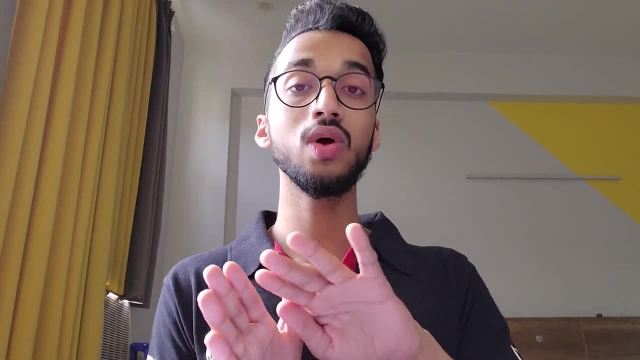 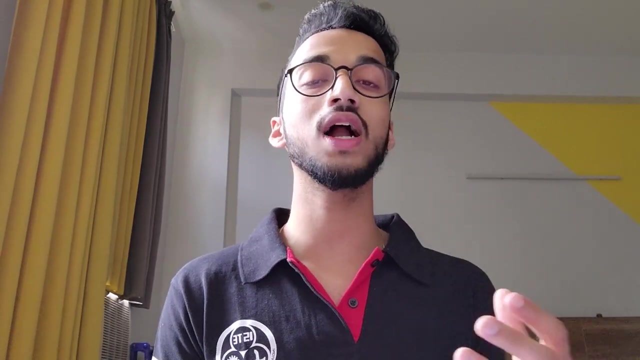 you would use to process images to train deep learning models. so that knowledge is important. so start with one or two frameworks and be proficient at that. now, when i talk about the software engineering part, right, that would require knowledge of docker and kubernetes and some cloud platform like aws and web frameworks and micro web frameworks like flask or 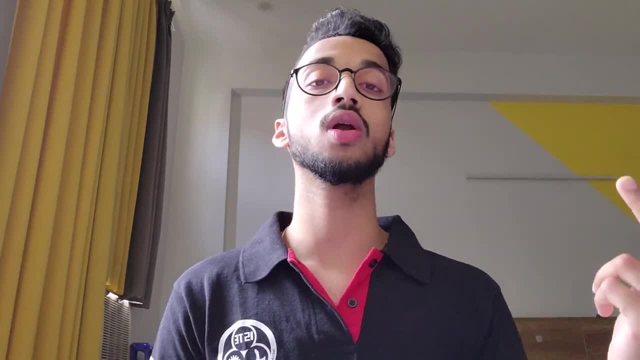 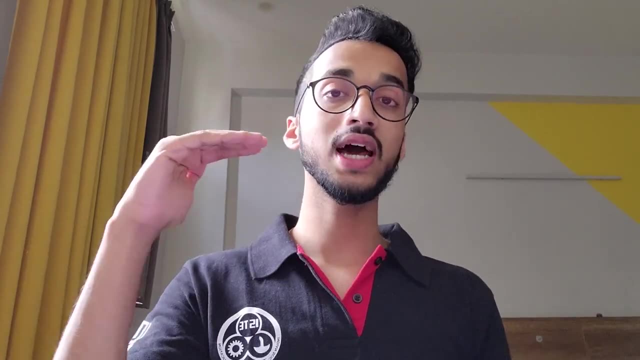 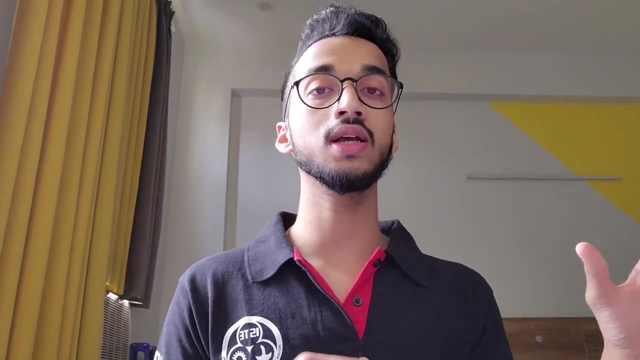 django. these are some things that you would need to push your model into production. so if you are a complete beginner and starting from scratch, i would recommend going step by step to target basics of machine learning, deep learning and computer vision right. do not directly skip to computer vision or directly skip to deep learning. start with machine learning first. right. so because 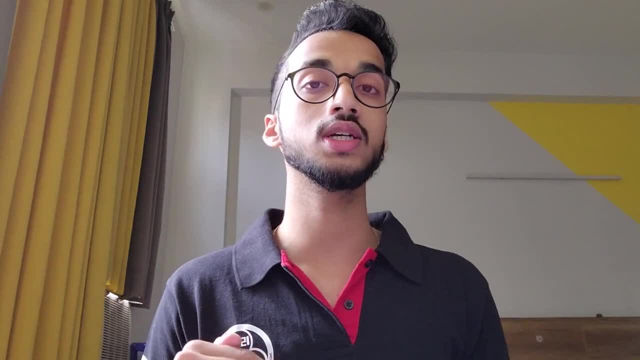 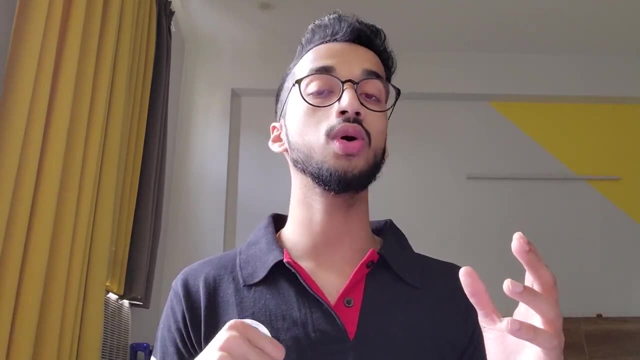 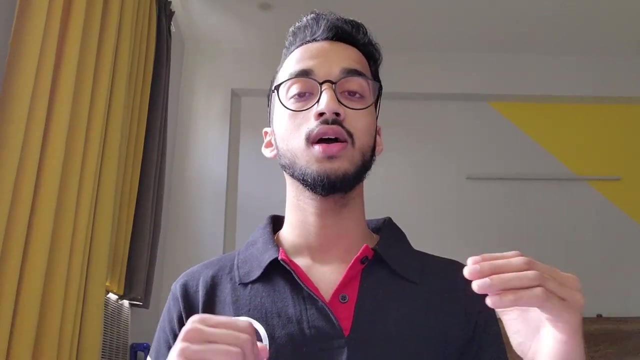 the basic algorithms of machine learning. let's say linear regression or lowest regression. these are the most fundamental. these are the most fundamental algorithms. without that, deep learning is going to be hard for you to understand or you wouldn't be able to understand that very clearly. next is, once you have the basics cleared, uh work on basic computer vision projects. 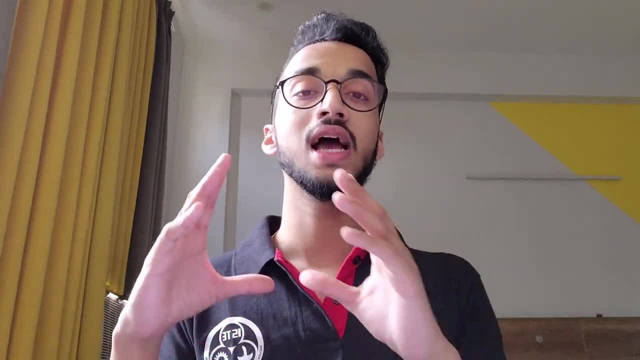 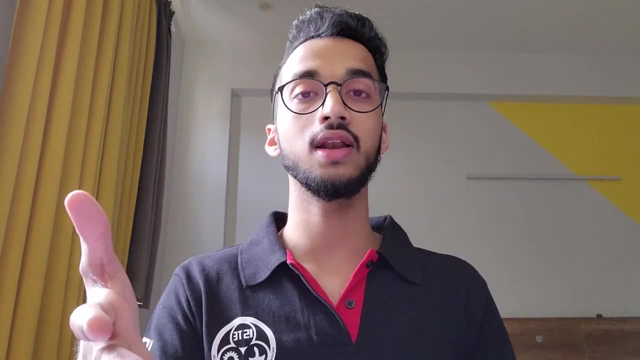 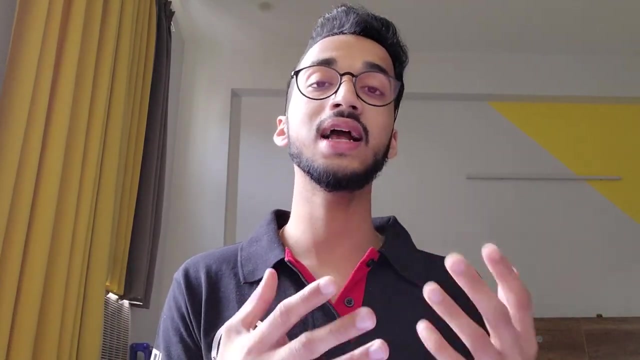 let's say the most basic project is is classifying handwritten digits. using the mnist data set you get an image of a handwritten widget. you predict if it's a 7 or a 4 or 10. right, that's a basic project. you move to more advanced projects. broadly, there are three types of problems, like classification, 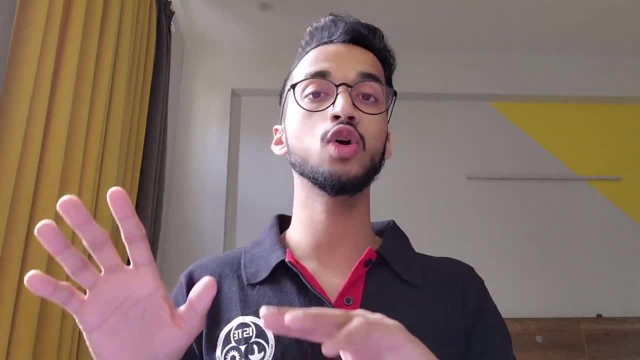 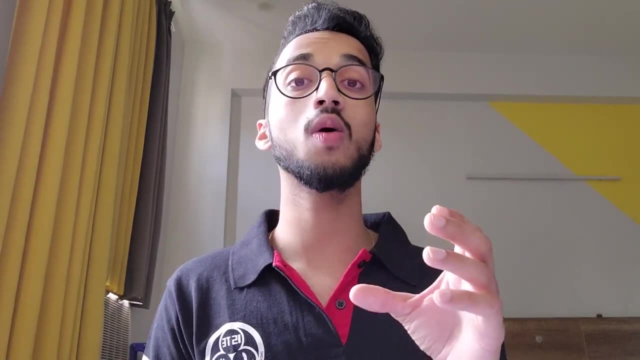 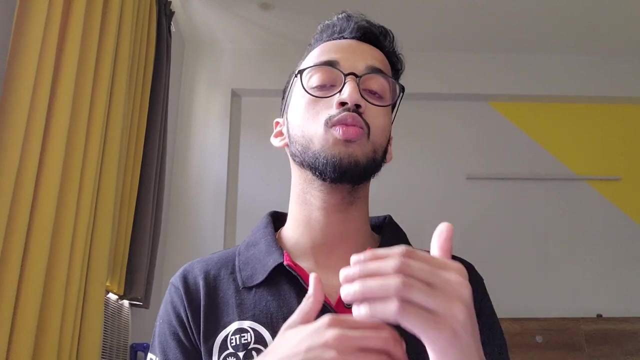 where you're basically distinguishing if it's a cat or dog or if it's a 7 or a 4 or the other. uh, other domain of problems is of object detection, where you're detecting objects in a frame, and lastly segmentation. so work on one domain and then slowly work on more and more projects and the